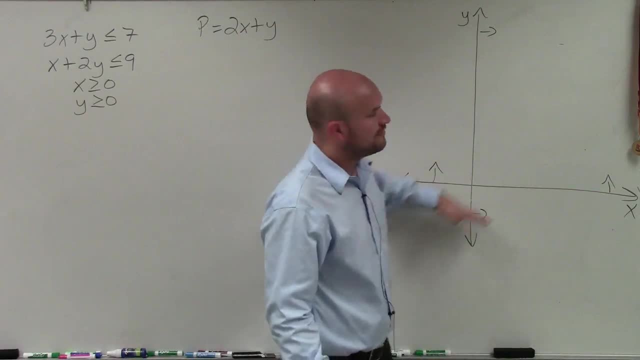 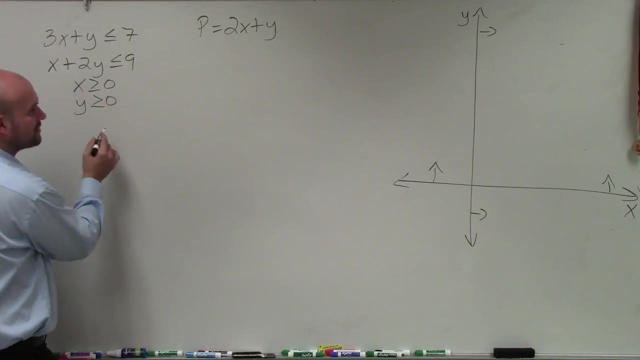 points to the right, y is greater than or equal to 0 is going to be your x-axis for points that are going up, because each of those axes are equal to 0. if you graph them Just like you'd graph: x equals 0, y equals 0, but now we're just pointing the arrows. 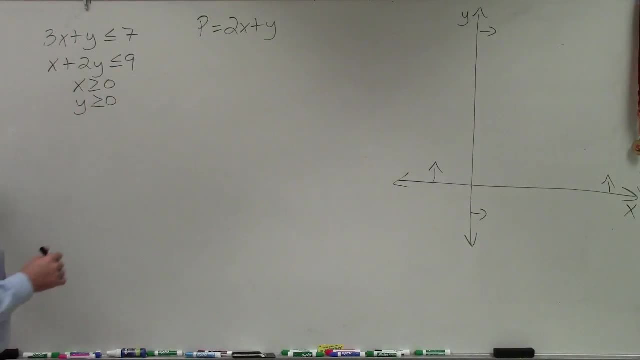 to what's going to make them sense. Then the next thing we need to do is now graph our other two constraints, which I have. 3x plus y is less than or equal to 7.. So to graph this, I'm simply just going to write this in our slope intercept form. So here I can. 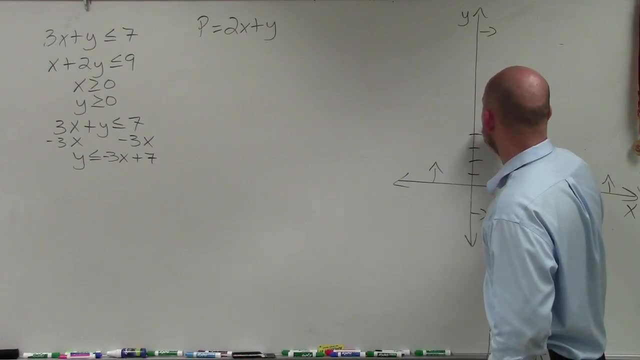 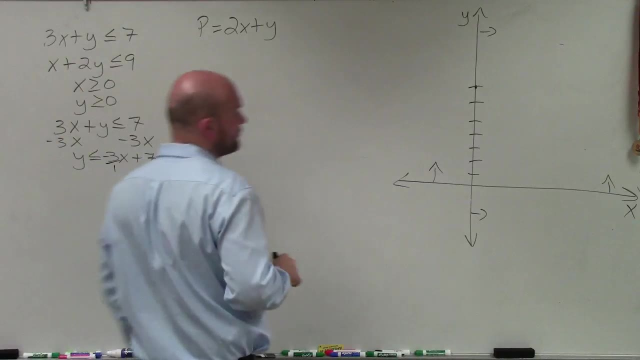 say, my y-axis is at 7.. So 1,, 2,, 3,, 4,, 5,, 6,, 7.. And then my slope is negative 3, so I can rewrite that as negative 3 over 1.. I'm going to want to graph this down towards my other. 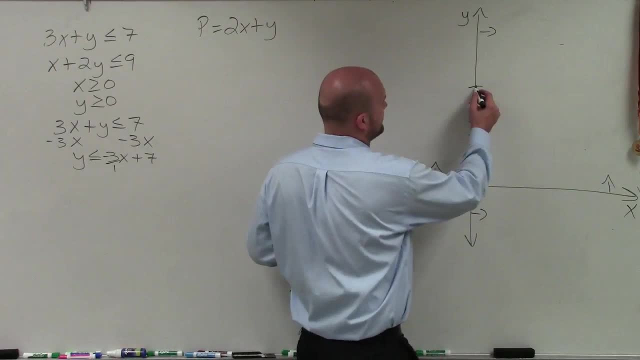 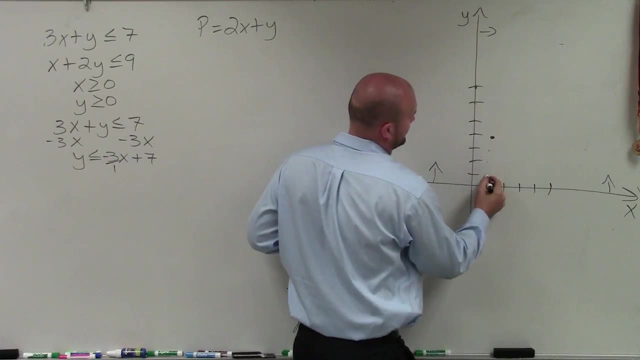 two constraints. So I'm going to go down 3, 1,, 2, 3, over 1.. So 1, 2, 3, over 1.. 1,, 2, 3, over 1.. 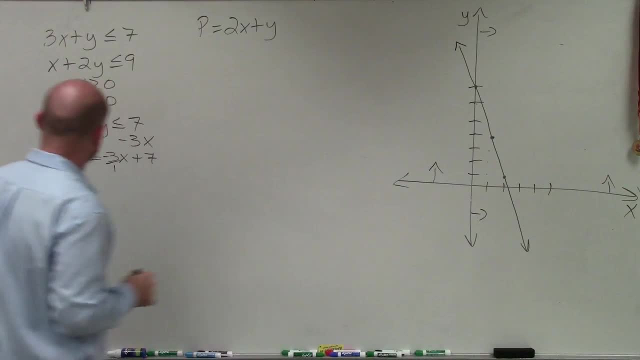 Oops, And then my next value here. the next equation is: x plus 2y is less than or equal to 9.. So now to go and graph that: I subtract the x here And I have: 2y is less than or. 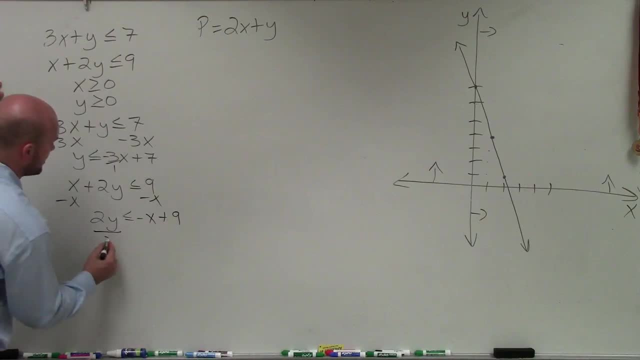 equal to negative x plus 9.. Now to solve for y. I'll divide that by 2y, So I'm going to divide by 2. And I get: y is less than or equal to negative 1 half x plus. I could do 9 halves. 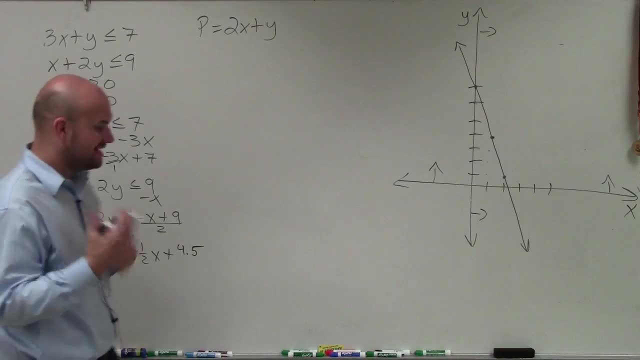 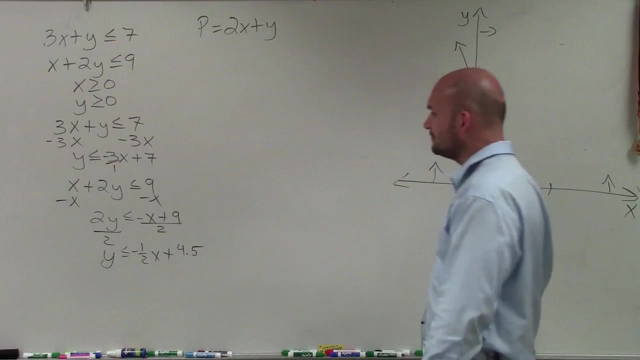 or I could rewrite that as 4.5.. And a lot of times I like to use decimals when graphing. even though I hate decimals, I like prefer keep thinking of fractions. A lot of times with graphing, it's helpful to know that, oh, my y-intercept is at 4.5.. 1,, 2,, 3,, 4,. 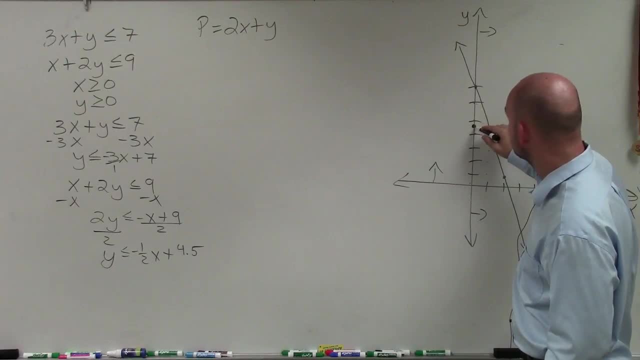 5. So 4.5 would be right in the middle. Now I'm just going to still. from there I'm going to go to the middle point of the next one over 1.. So I'm going to go to the middle point. 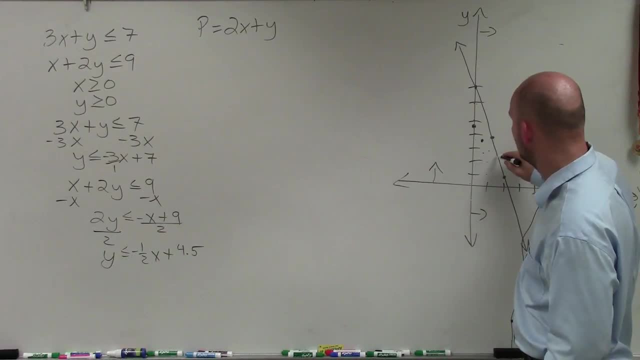 of the next one over 1.. So I'm going to go to the middle point of the next one over: 1.. Middle point of the next line over 2.. Down: 1.. Oh, it should be like over there. Middle point of the next one down: 1.. Middle point of the next one down: 1.. Oh, over 2.. Why did 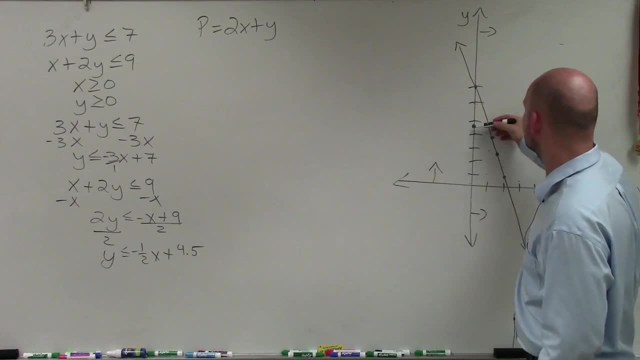 I not do that, All right. So down 1 over 2.. 1, 2. Down 1.. Down 1 over 2.. Down 1.. Down 1 over 2.. Down 1 over 2.. And then down 1.. Down 1 over 2.. 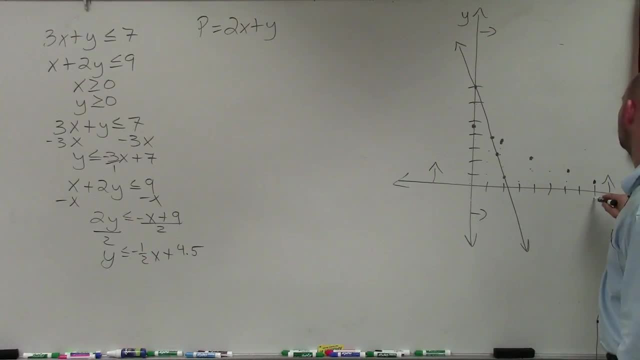 Wow, My graph is really far off here. And let's go ahead and see: These are all x's less than or equal to this one. And then let's go ahead and see: These are all x's less than or equal to this one, And then down 1 over 2.. And then let's go ahead and see These: 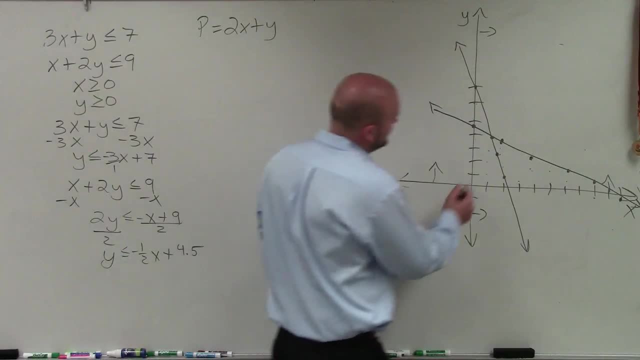 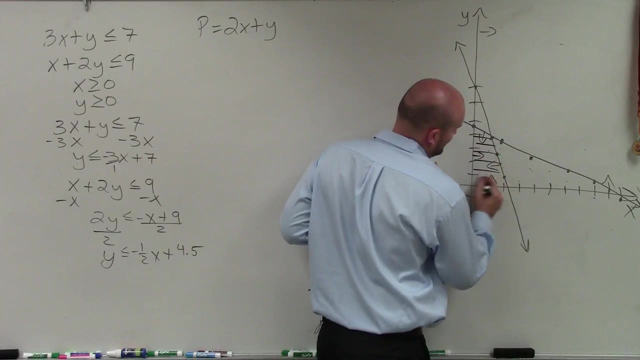 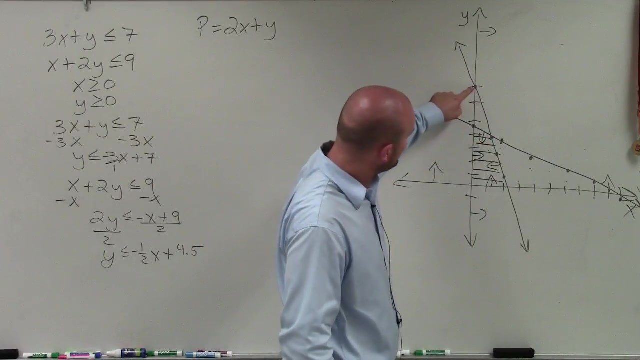 and this one was y is less than or equal to, So therefore I'm dealing with these two boundary lines are going to provide me with this feasible region, which is right inside of here. So, basically, I need to make sure I can determine what this- you know- point is that they're intersecting at, and it looks like per my 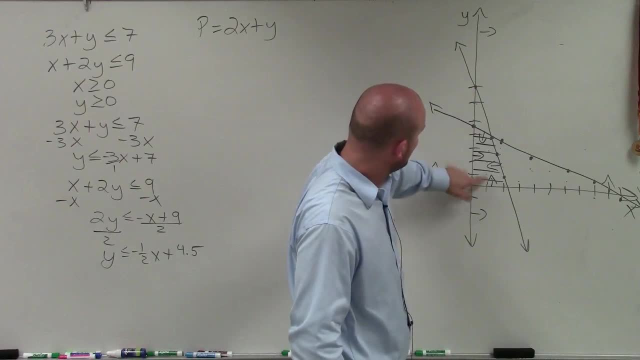 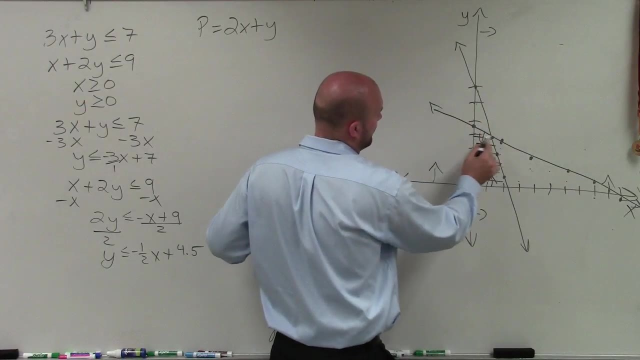 graph. that's at the point seven. so that'd be over one over one, two three down three over one. so that's looks at that, the point six. five four, one, so one comma four. So let's just verify that's a point for both of these negative twelve. 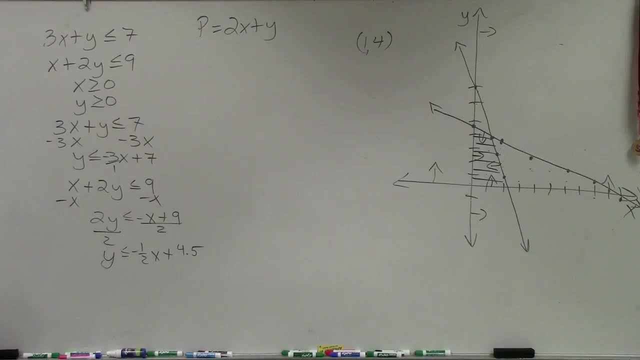 that's going to be five and one. oh, four comma one. no, one comma four. So I put in a one four that works for that one. yes, So to verify this point, I'm going to put in a one four that works for that one. yes, So to verify this point. 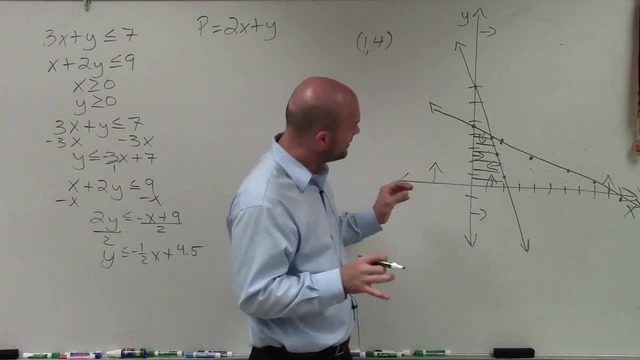 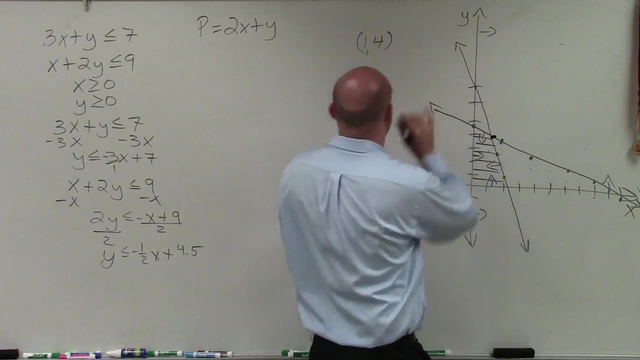 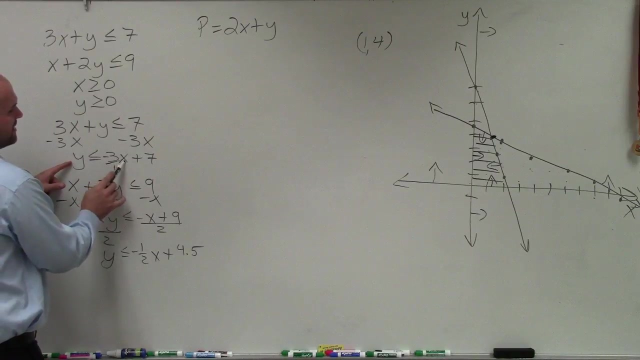 even though, like like I said, my graph is really really off right here. per my graph, this point is at one comma four. Now if I plug in a one in for x, I have negative three times one, negative one, two negative three times one, which is negative three plus seven is four, and then the y-coordinate is four, so four is. 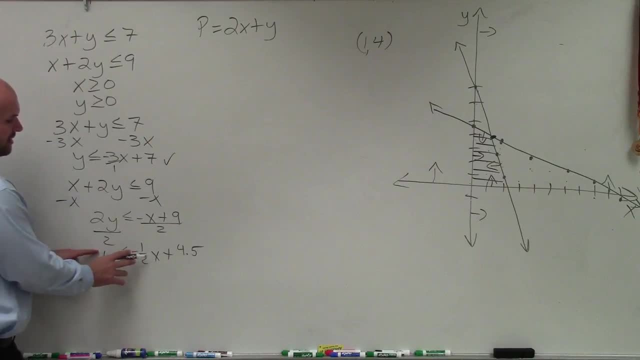 less than or equal to four. so it works. If I plug it into here. I plug in a one negative, one half times. one is negative, one half or negative point. five plus four is four. again four is y is four. so then four is less than or equal to four. so 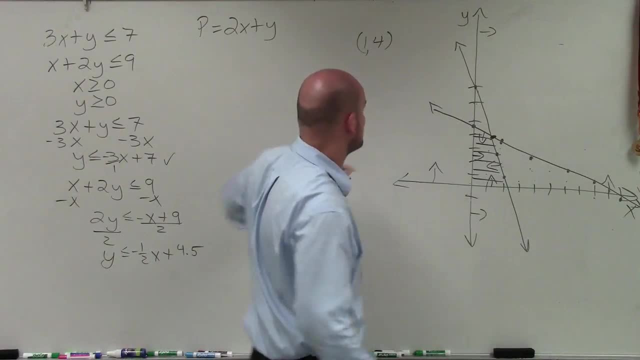 that point works. The next one here is my y-intercept, which is at four point five. so I'll write four point five, comma zero. and this next one is: I'm going to be following this line here. so if I go down down, three, one, two, three over one down. 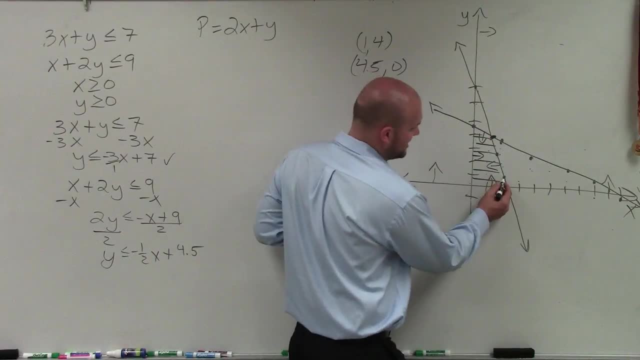 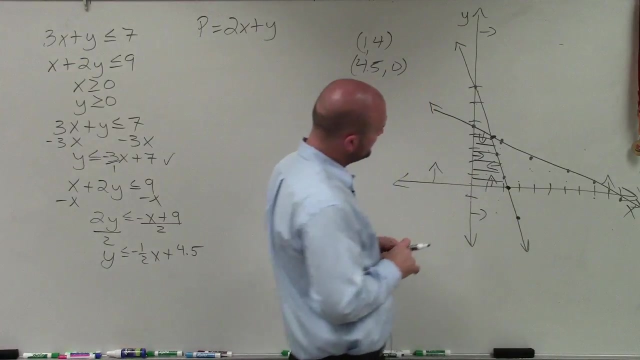 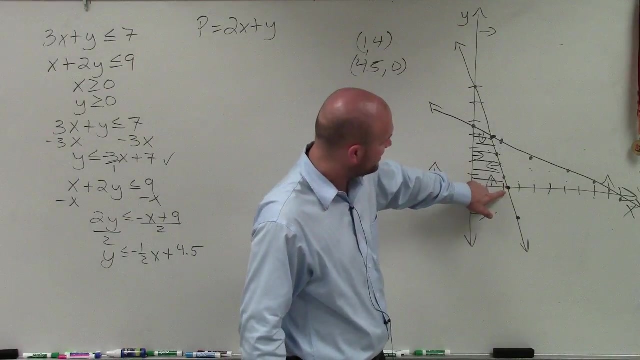 three. one, two, three over one. Now for the next point. I'd go down through again: one, two, three over one. So it's between one, two and three. so it's between two and three. So the way I can identify what exactly that point is is that point is when x is equal to zero. so 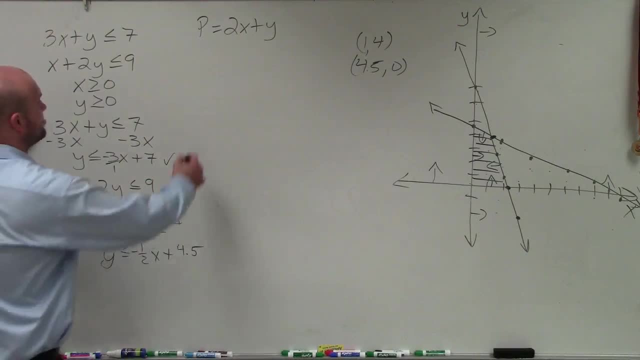 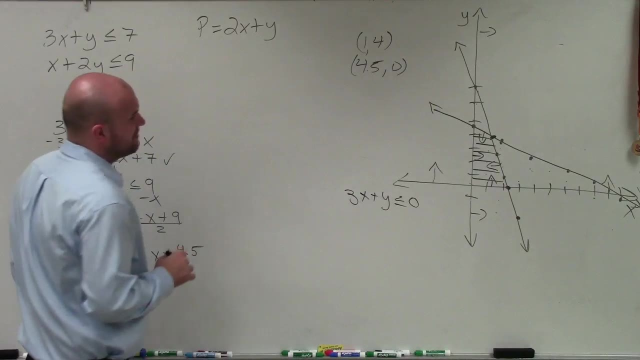 I'm going to go back to this equation that produced that line, where I have the three: x plus y is less than or equal to zero. I'm going to say, all right, well, what about when my x value is equal to seven? what about, or not, when? 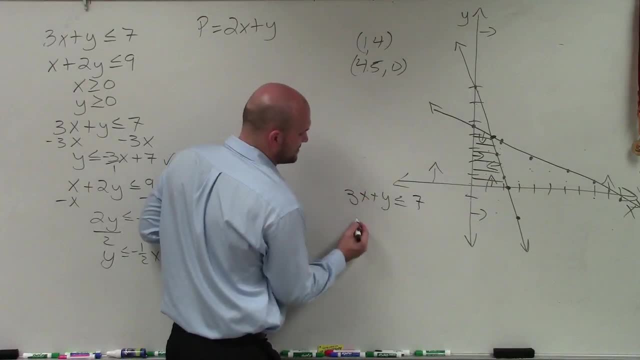 zero. I'm sorry when my y is equal to seven or my y is equal to zero. so I'll do three times x plus zero is less than or equal to seven. and then three x is less than or equal to seven. divide by three: divide by three x is less than or. 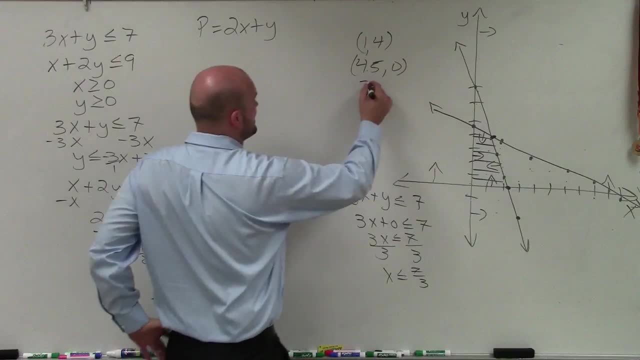 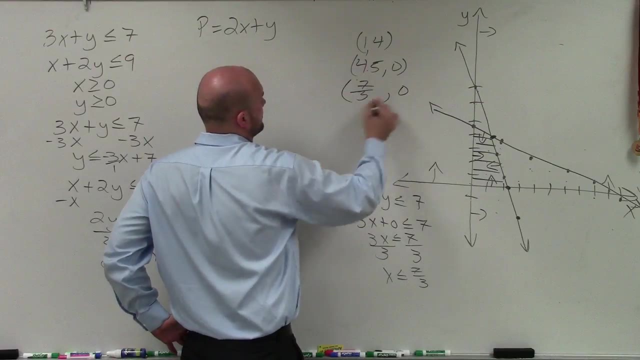 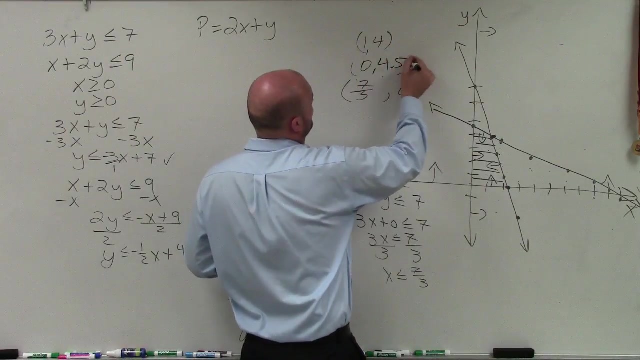 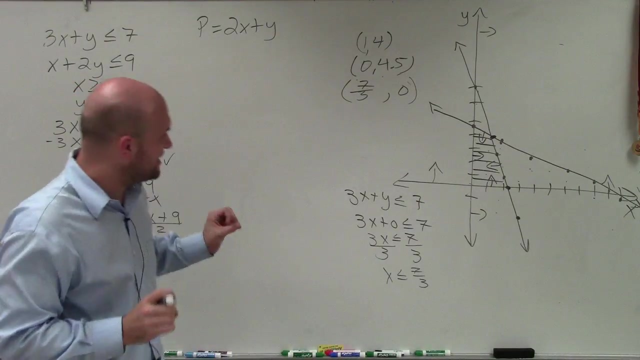 equal to seven-thirds, So my x-coordinate is seven-thirds comma zero. Oh, I wrote that wrong. sorry about that. Okay, so now let's go ahead and determine. my apologies take a little while, but hopefully you guys understand. you know when you're dealing with, when you're dealing with fractions- a lot of. 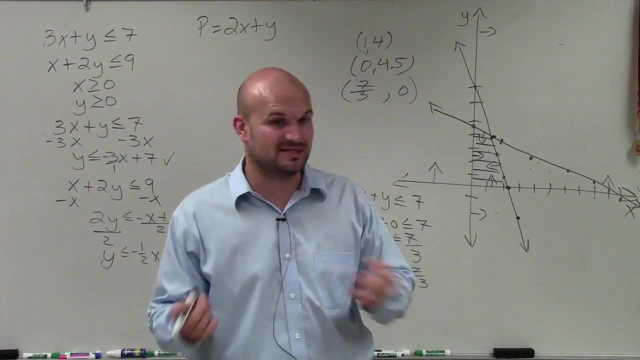 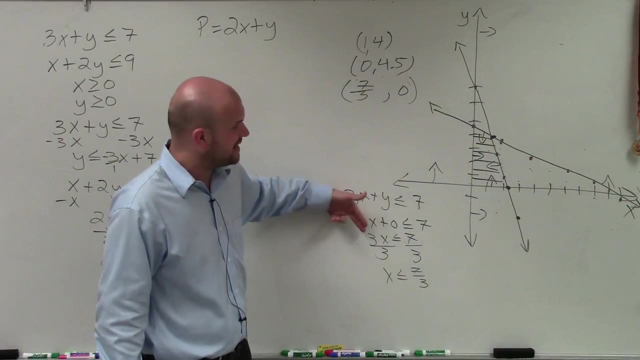 times, you know, especially when you're dealing with your graph, or sometimes it can be, you know, is this right or wrong? I can always determine. what is that point? well, that's the y-intercept. so I plugged y zero in for y into that equation of that constraint line, to be able to determine what the x value was. The same. 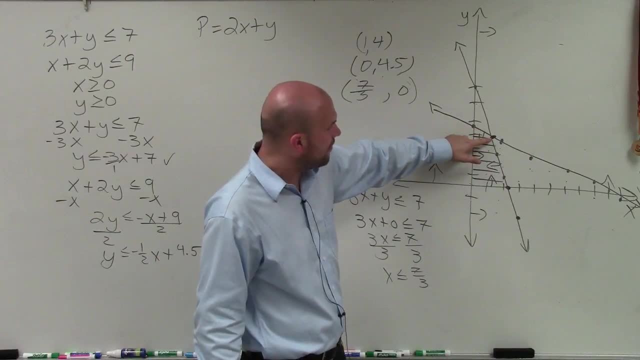 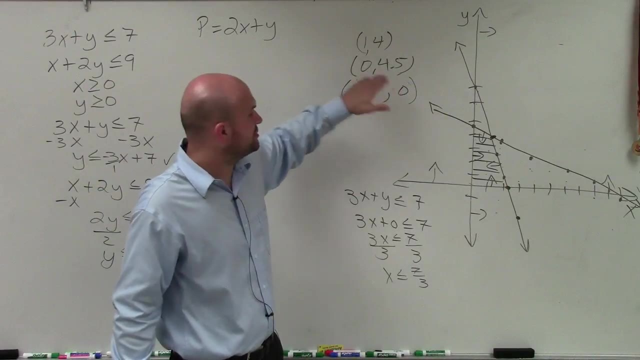 thing here. you know, I was pretty sure the coordinate was one comma four, but to verify I plugged in x and y into both of those equations to make sure it worked. and then this one I just rewrote should be: x zero y is 4.5.. So now let's go and